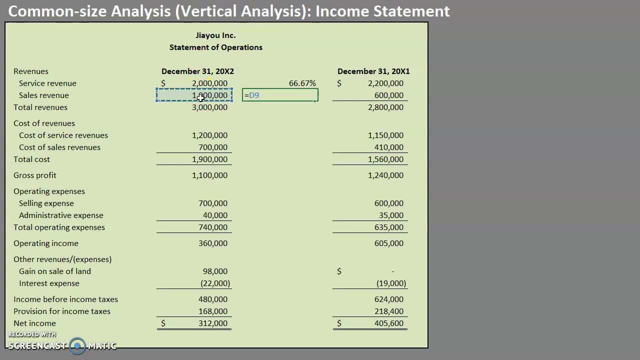 next one here. So for sales revenue it is going to be a third, 33.33%, And we are going to continue to do that for every single line item. And now I know this isn't an Excel video, but just so that. 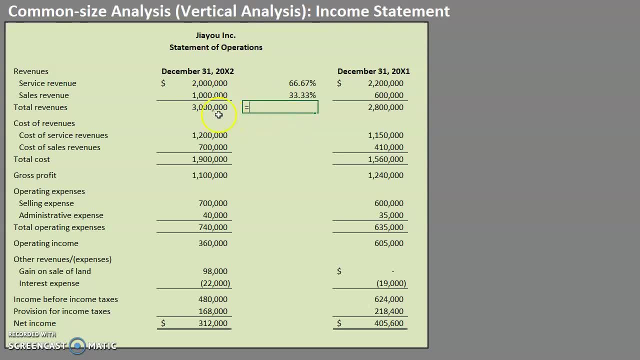 you can kind of see I'm going to be using a formula to help me. go ahead and copy this formula down so I don't have to go one by one. Notice that for every single line item on here, I want my denominator to stay constant at 3 million, so I want it to stay in row 10.. So I'm going to use an. 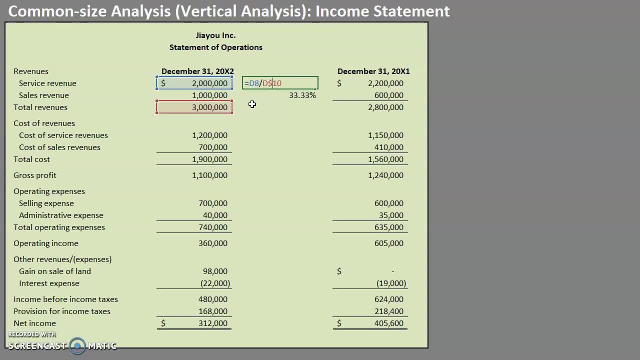 absolute. Hopefully you've seen these before. That will keep my formula consistent in d10 as I drag down. So, for example, let me just do these first three. you'll see now when we look at it, it stayed with d10. I did this one too, d10. let's go ahead and drag it all the way down using our fill handle. 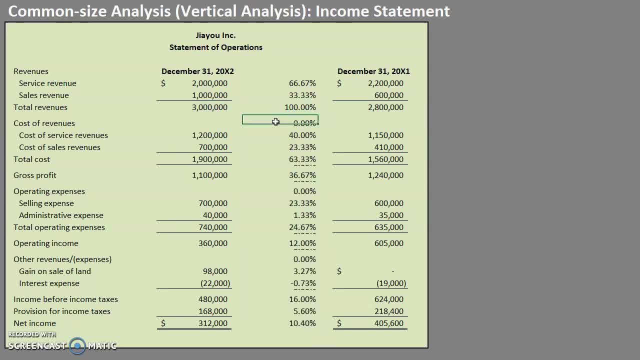 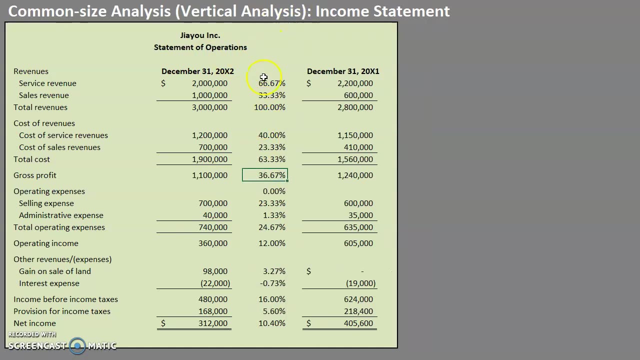 there we go now. there will be a few zeros that I have to delete as I go through this, but for the most part it did almost all of the work for me. there we go. so now, when you're taking a look at this information, you can kind of see here: 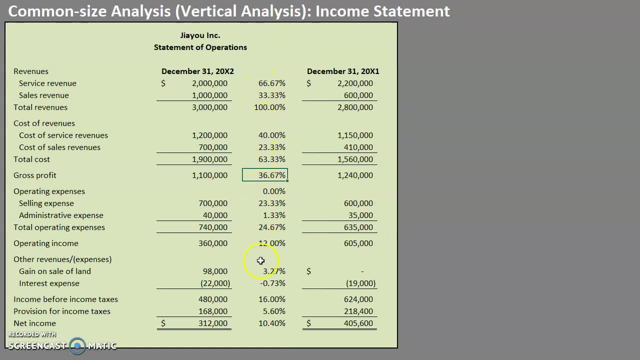 when we are analyzing our net income, we can see that net income ends up being 10.40 percent of our total revenues, and it usually is good practice to go ahead and put your math lines in the same way you would for the regular line items that you're seeing right next to it. 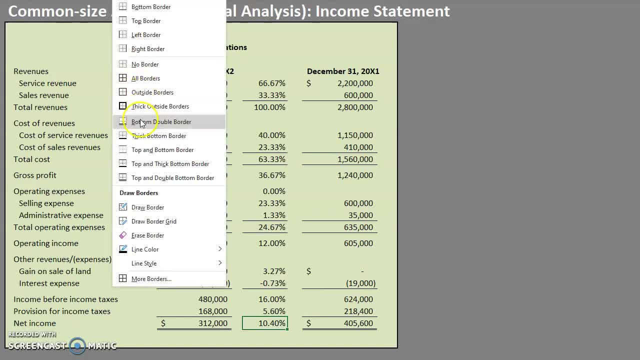 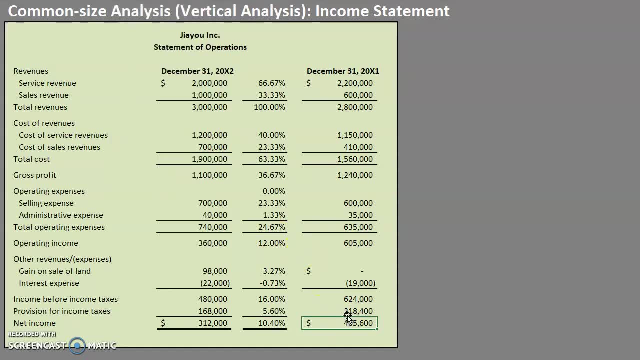 so just to kind of clean it up a little bit, there we go. so, as you can see, the purpose of doing this is to essentially kind of grab and see how much of our total revenues each cost is eating up and then also how much we're left with at the very end. for 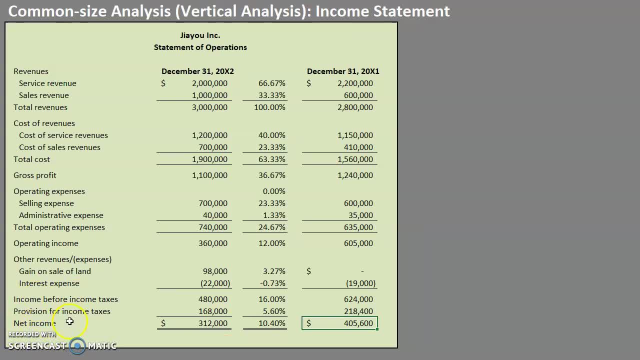 our net item, so our like our net income, our income before income taxes, operating income, gross profit, so on and so forth. I'm going to go over here and I'm going to quickly do one for this side as well. so remember, I'm doing every line item with the denominator of revenues. so here is my revenue.